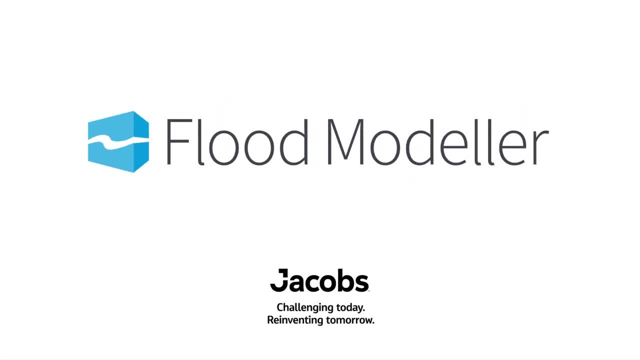 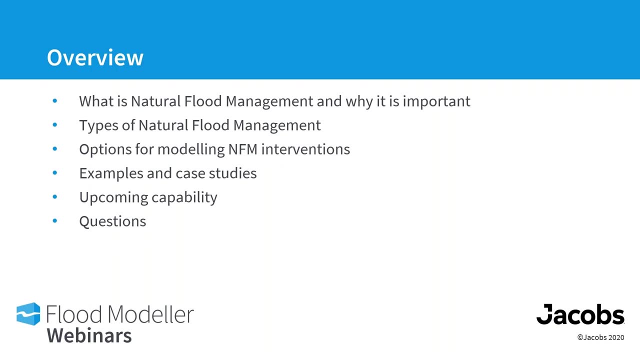 Just give you an overview of what we'll be talking about. So the first one we'll look at is: what is natural flood management? What do we mean when we say NFM, and why is it important? I'll look at the different types of NFM intervention that are currently being considered and how. 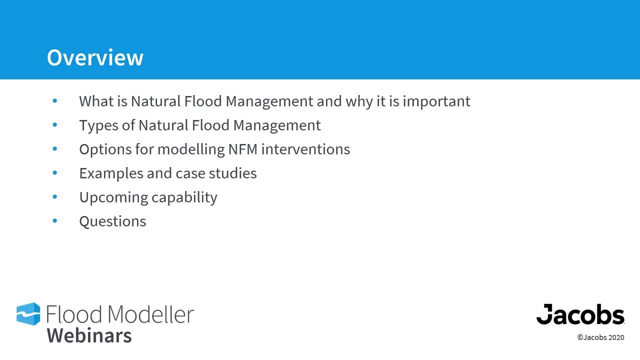 they can affect channel flows. I'll spend the majority of time looking at options for modelling NFM interventions using a number of case studies and examples. So once we've identified an option, how do we actually test that within the model and evaluate its benefits? 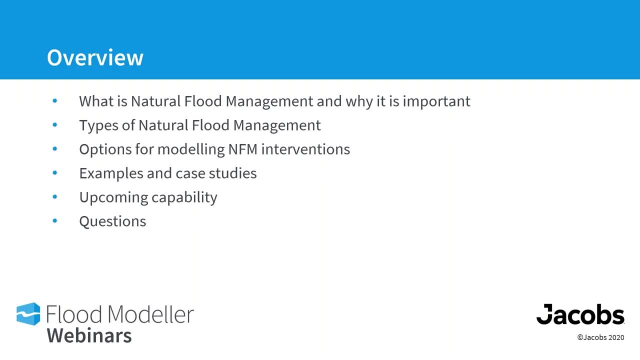 Towards the end, we'll look at some of the upcoming functionality within flood modellers, so the new functionality that's coming in future releases and how that can further enable us to consider NFM and other options. And finally, we'll have time for a few questions. 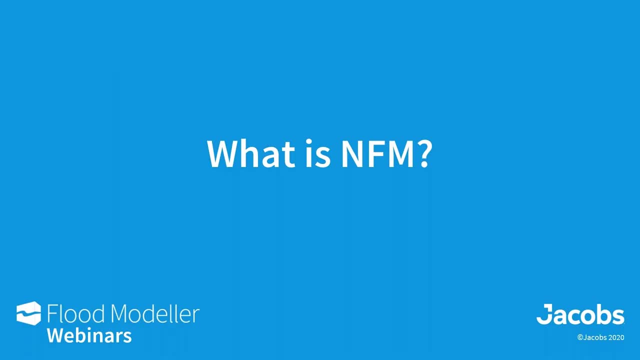 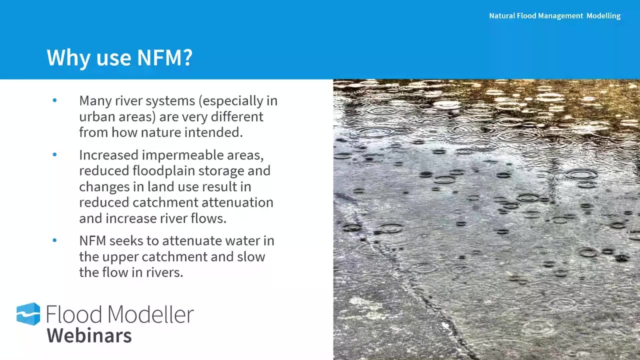 towards the end of the presentation, Focusing first: what is natural flood management? What do we mean when we say NFM? So, as I'm sure you're aware, many of you know of Kaf, những situations where we use flooding block systems, toてch. 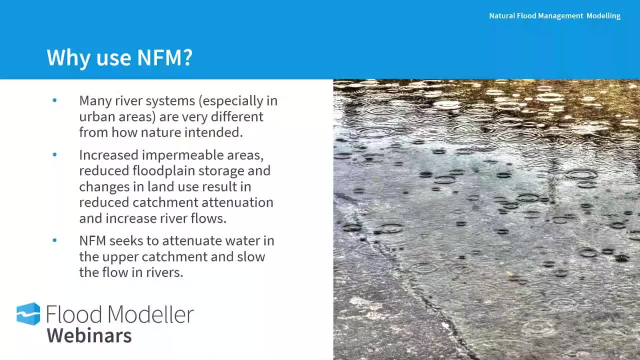 regimes, but at the same time, we are looking at adding flood block systems to your road planning drive. what is exactly that? even if only rainy season or dams become more difficult than winter in terms of water treatment or対象 water. Focusing on that and actually will also look at how we can workrà between sustainability and mineral data processing, and what doğa kelngewelearning will look like and how can we use observational studies to help sogarneutrically parse up the requirements. So we do have the three areas that he's interested. 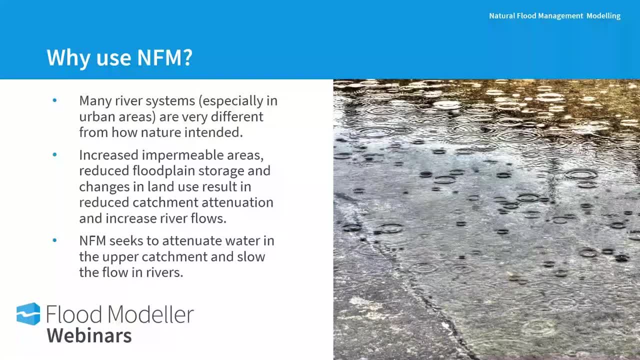 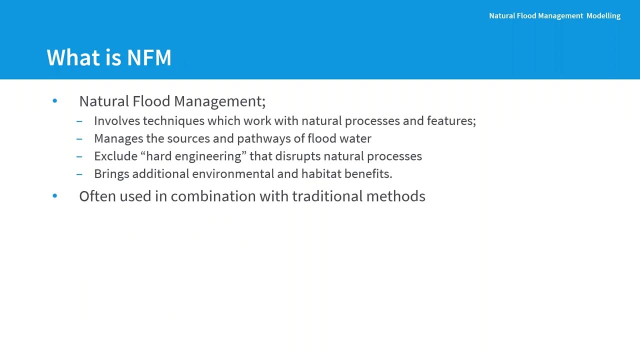 catchments and, as a result, increased flows within rivers. NFM seeks to attenuate water in the catchments in the upper catchment more and slow the flow of water in our rivers, thereby reducing flood risk as well as bringing environmental benefits. NFM techniques looks to use techniques. 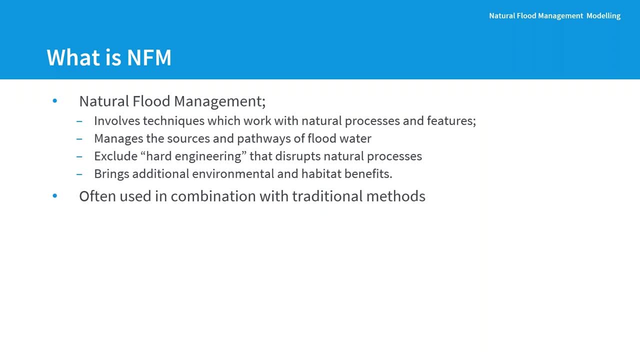 which work with natural processes and features to enhance flood risk benefits: Managing sources, so where the water's coming from, and the pathways, the rivers which water flows to get to our receptors, to our urban areas. NFM looks to exclude hard engineering options. 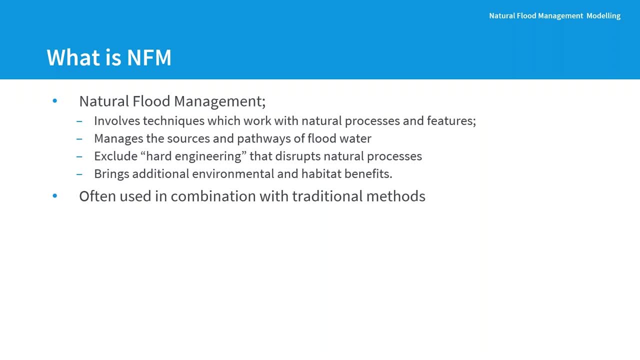 which disrupt natural processes and, as well as bringing flood risk management benefits, bring substantial environmental benefits. So, as well as reducing flood risk, we're increasing habitats, creating new environmental areas with associated benefits. Increasingly, we're looking to combine both NFM with more traditional methods. 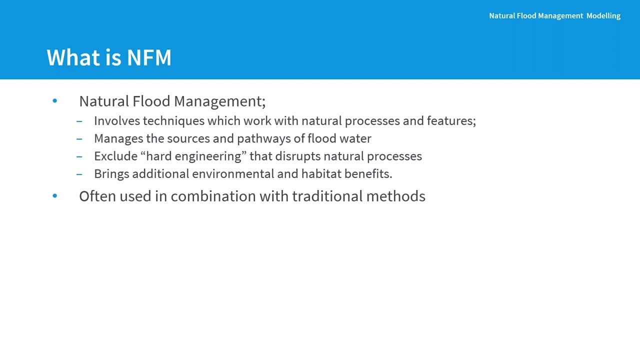 So, for example, if you're building a traditional linear flood defense, a flood wall, through an urban area, you may be able to achieve a given standard of protection with that wall. But if you combine that with NFM in the catchment upstream, 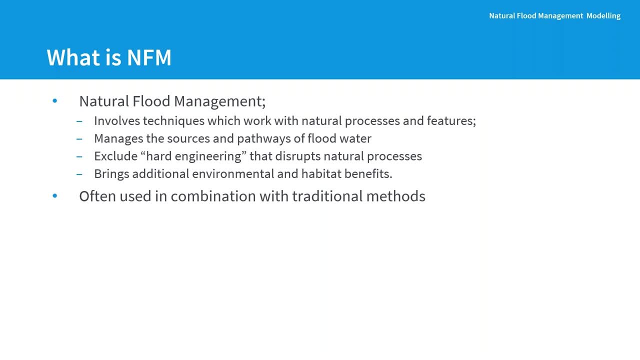 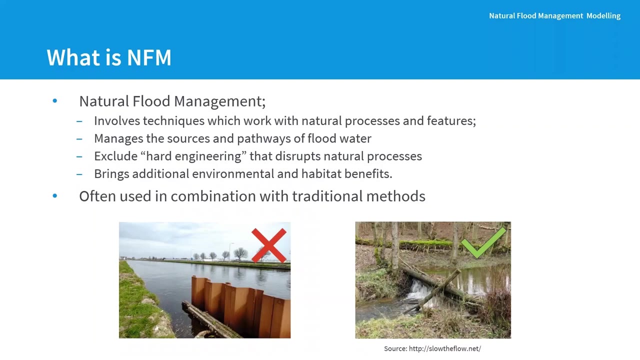 you can increase the standard protection your defense is offering you, as well as allow it adaptation for climate change. So, in summary, we're looking for less of this and more of this sort of approach. So less hard engineering and more natural process engineering. example: 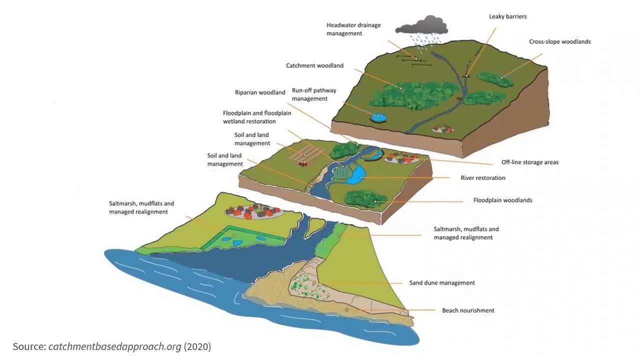 but we're going to move over to the next slide. It's definitely a little bit more complex than what you're seeing here in the right hand side. So what options does NFM encompass? This is an image from the catchment based approach website. 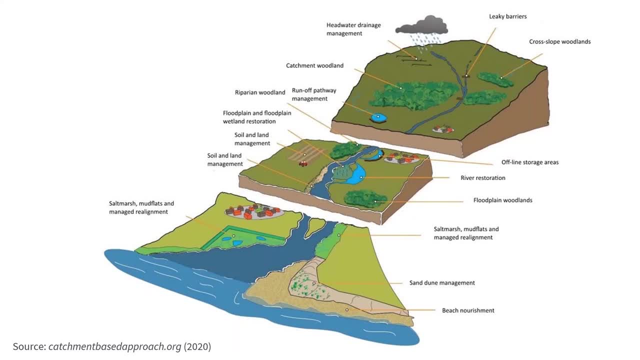 which captures quite a few of the the options being looked at. It's divided into the upper, mid and lower catchments, And so in the upper catchment you've got a number of options which try to attenuate water in the catchment. 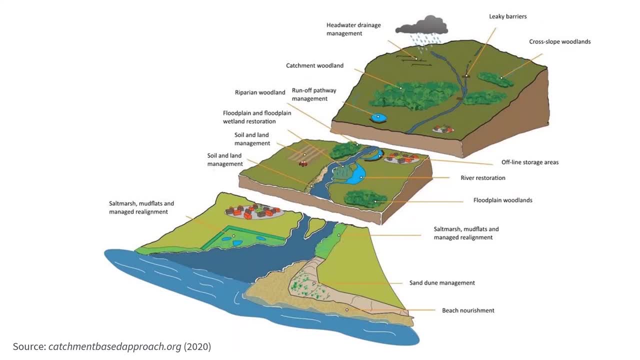 So keep water in the upper catchment rather than having it flow directly downstream and causing a flood risk. So you've got things like headwater drainage management. this could be things such as peatland restoration: reducing the drainage out of peatland areas. 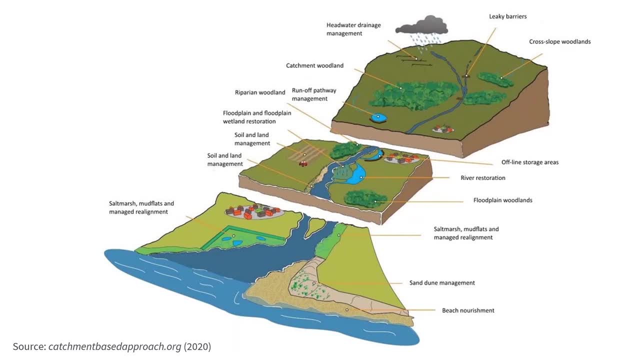 planting up woodlands, so woodlands are great for reducing flowing rivers. they create depressional storage. if you're in a woodland after a rainstorm, you've got lots of water stored in in the root areas of trees, on the surface and the undulating ground, as well as increasing infiltration of water. 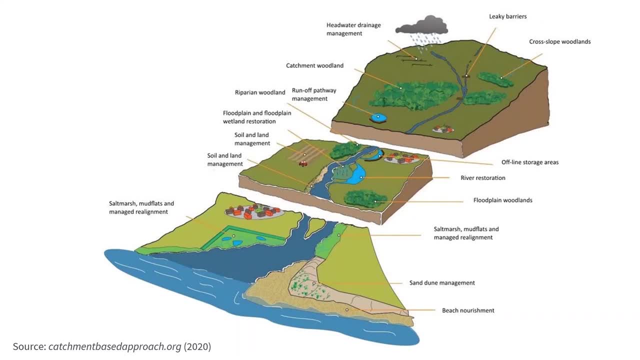 and transpiration of water. options such as leaky dams, which we'll look at in a bit more detail later, hold water back in the river, so creating localized areas of attenuation. in the middle caption, we've got options such as river and floodplain restoration. so, returning 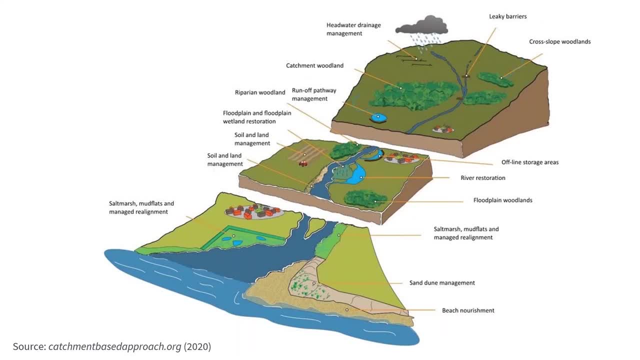 rivers to their natural courses, increasing meanders and reconnecting floodplain storage areas to the river. often, floodplains are detached from the river by embankments and other features, and by reattaching these we significantly increase attenuation and you can create new offline storage areas, so wetland areas, bringing both environmental and flood-resistant. 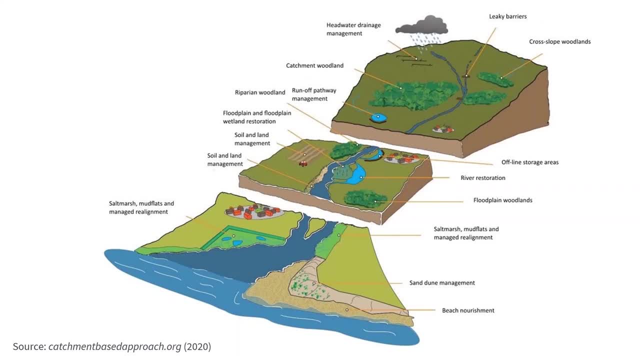 benefits. Combined with this, we have soil management options, so simple things like plowing fields in different directions can have a significant impact on how a catchment responds and reduce flood risk. downstream, As we go further downstream towards more estuarine areas, we've got things like realignments, so where we create salt marshes and mud flats. 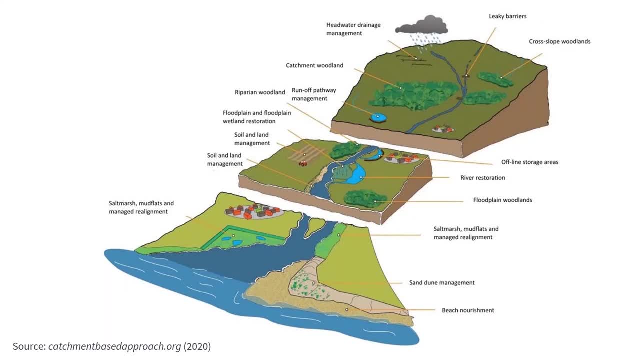 as well as sand dune and beach nourishment options, to again bring both environmental and flood risk benefits. On paper, these things sound reasonable and they seem like they would provide a flood risk benefit, but in order to justify investment in NFM, we're often asked to demonstrate and evaluate how effective they would be so to spend, you know, a? 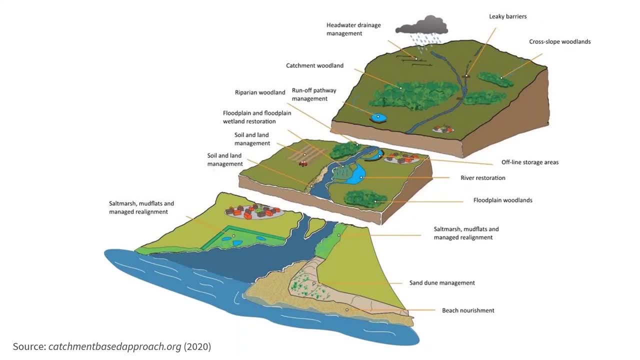 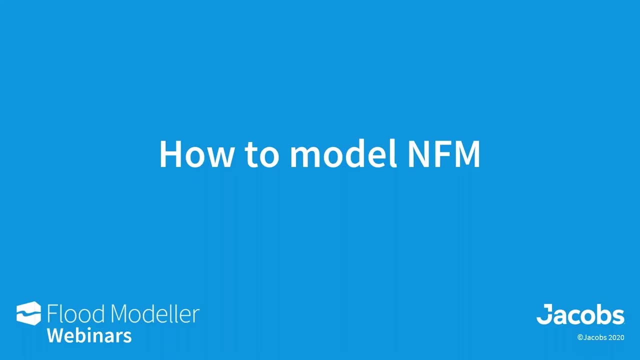 million pounds on on planting up woodlands or adding in leaky dams. how much benefit will that bring me, both environmentally and from a flood risk perspective? and to evaluate these options, we need to model them in some way. we need tools in which to evaluate their benefits. 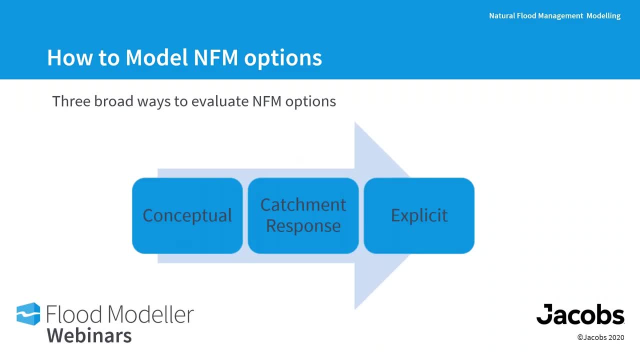 I've I've divided these modeling options into three broad categories and there's there's obviously a lot of overlap between them, but broadly we've got to start. we've got conceptual modeling, so conceptual analysis. this is usually things like opportunity mapping, so we can use GIS data, spatial data, land use data to try identifying the types of NFM opportunities. 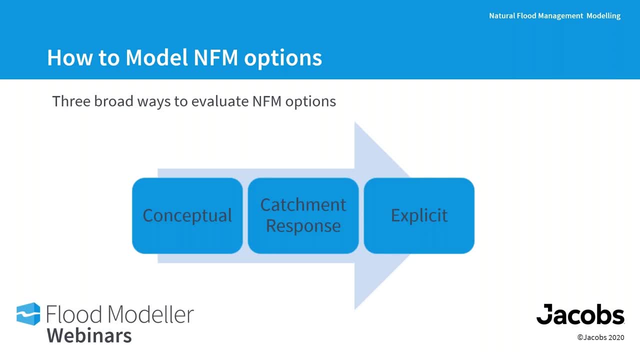 which may be relevant within the catchments, and I'll talk about this a bit shortly. So by doing opportunity mapping we can identify the types of NFM which may be available to us before we even start doing any modeling. We can then look at catchment response modeling broadly. this can be: 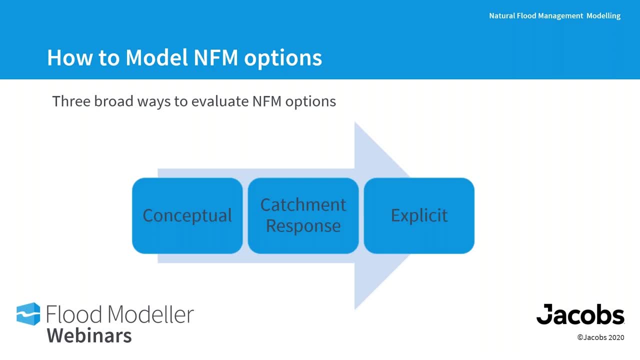 divided into two types. so we've got sort of conceptual catchment modeling using rainfall runoff models such as SCS and RFH, where we change the parameters within our catchment models to represent NFM, so we reduce urbanization or increase infiltration, for instance, to represent 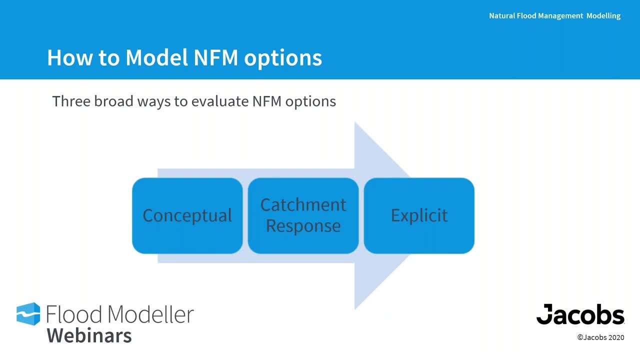 increased NFM within the catchments, Or we can do the more complex direct rain on grid type modeling. this is where we build big 2D models of our catchments. we drop rainfall directly onto it and we model the different processes that are going on within that catchment and finally we have explicit modeling of NFM. 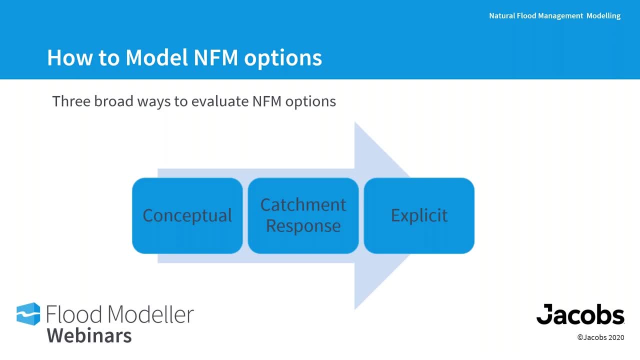 features. so using a 1D or 1D- 2D models to explicitly model those features that may be putting leaky dams in a 1D model or modeling floodplain reconnection with the 2D model, for instance. I'll talk through some of these models later. 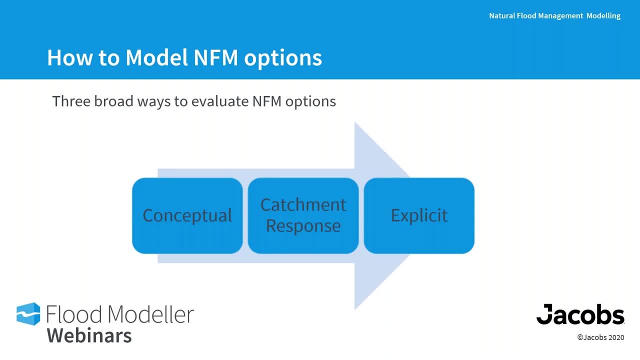 So I'll talk through some of these models later. And I'll talk through some of these models later. And I'll talk through some of these models later. And I'll talk through some examples of each of these different options in the next couple of slides and what their benefits and challenges associated with them are. 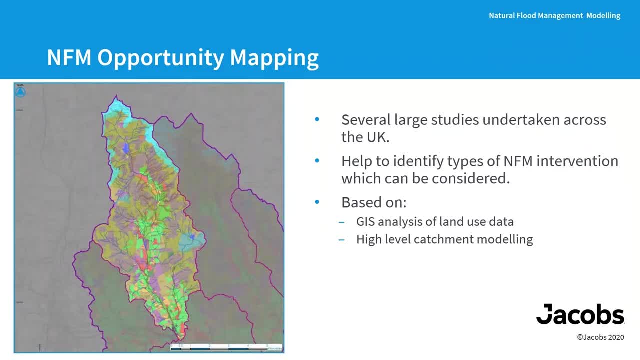 So the first example is opportunity mapping. this is an example from the Rivers Trust, from their Cumbria opportunities mapping from a few years ago, and this is one of several large studies taken across the UK and elsewhere, and so using GIS data, land use data, we can look across a 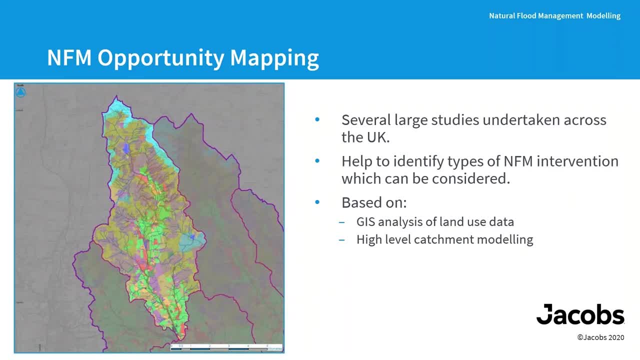 couple of different sites and we can money map a particular site at a different time and we can see the real benefit of this data and we can also see the risk of this data being affected. and we can see the real benefit of this data and we can also see the biggest risk of this data being affected. 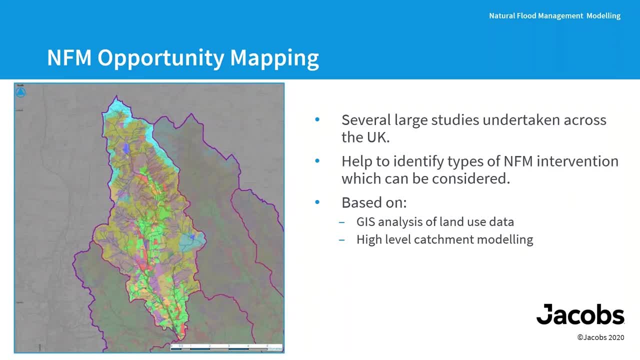 by the impacts of the natural disasters. So do the catchments lend themselves to changes in lands use, additional forestation? are there peatland areas which could be benefit from restoration? does the catchment gradient slopes lend themselves to things like leaky dams? and so, by evaluating these things at a high level, we can start to eliminate options or 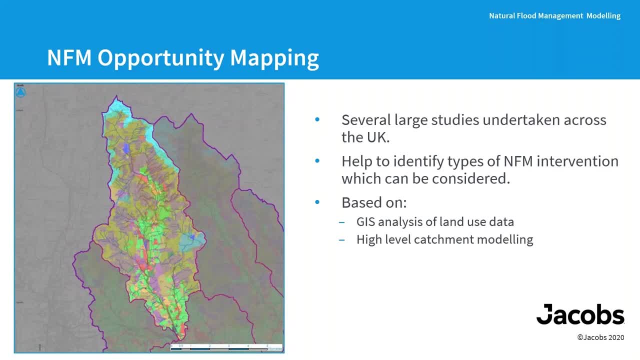 identify options which can take forward to further investigation, and these opportunity maps could also be accompanied by some high level camera authentication so that we can move forward to the next stage of the research- catchment modeling- to to try and identify not just what sort of options could be considered. 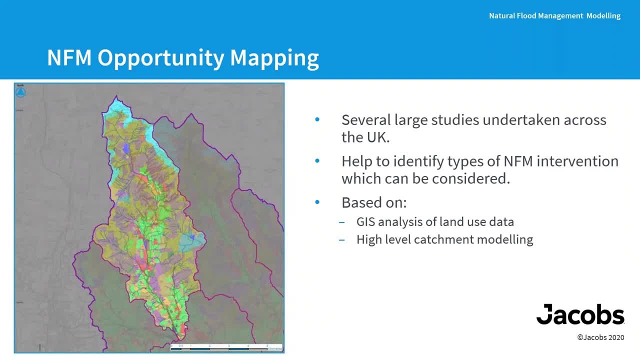 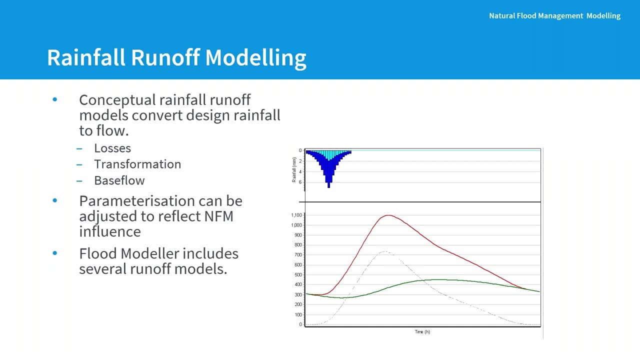 but also in a high level state, what sort of benefits they would bring. so, moving on to catchment modeling, the first thing you can consider is use of conceptual catchment models. these are things like rainfall runoff models, and there are quite a few of these built directly into blood modeler. so these conceptual rainfall rough models, uh, divided. 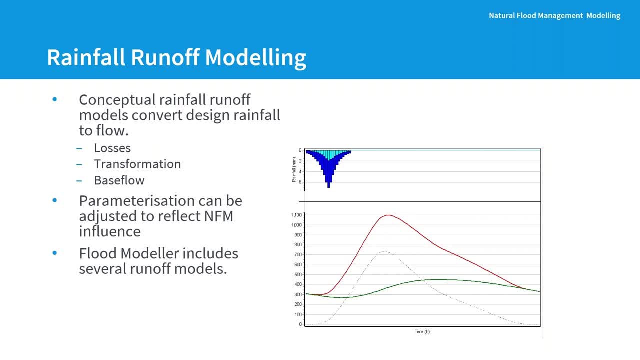 into several sub elements. uh, we've got the direct rainfall. so, um, on the image on the right hand side, this is output from a rainfall rough model from flood modeler and we've got the. the blue height graph at the top is the input: rainfall. we consider rainfall losses, so how much of that water? 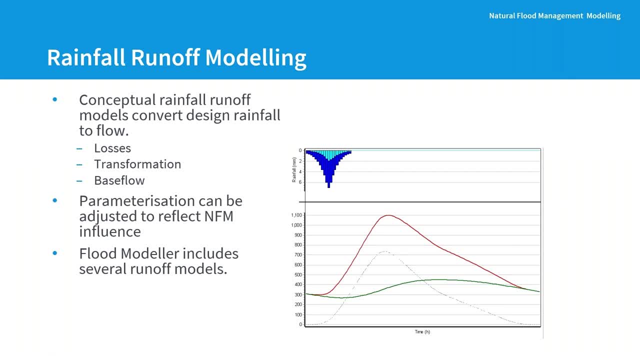 is infiltrated directly into the catchment. we look at transformation so that the water that didn't infiltrate and runs across the surface. how long does that take to get from one end of the catchment to the other? that's usually a unit hydrograph approach. 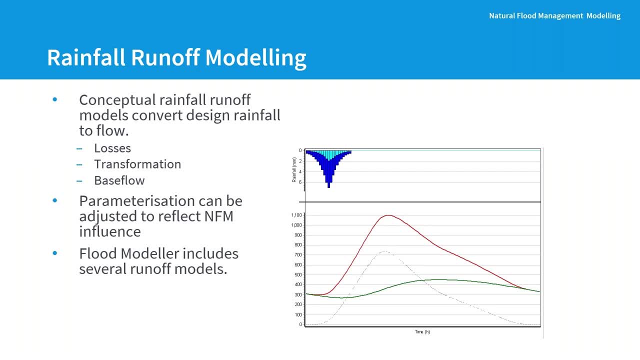 and then we've got the base flow component. so this is the subsurface hydrology, and we use parameters to describe how these different sub models behave, and we can adjust these parameters to reflect nfm intervention. so it may be we increase infiltration or we we reduce the amount of urbanization within the catchment, for instance. we change the parameters. 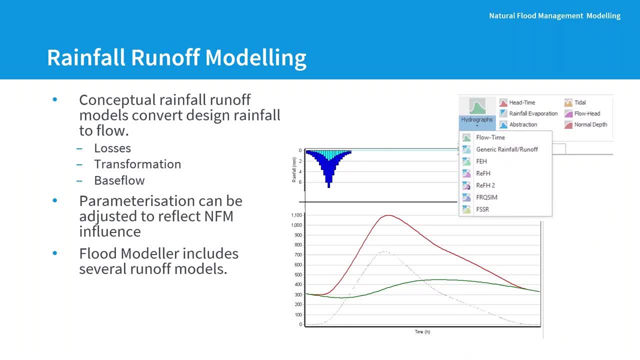 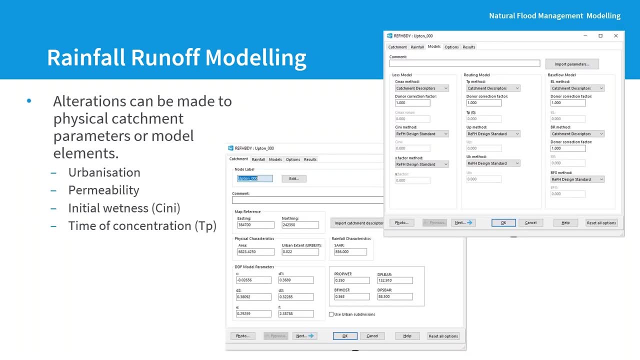 as i say, flood model is quite a few of these models built directly into it, so you can add these directly into your hydraulic model. the one here is rfh, but one another one worth, uh sorry. and by changing the the parameters with these models we can adjust how the catchment behaves. so it may be, for instance, you change: 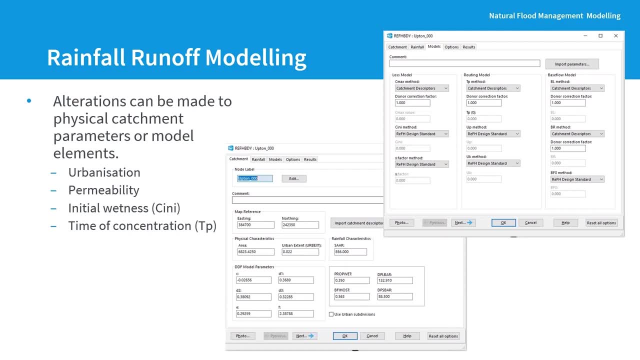 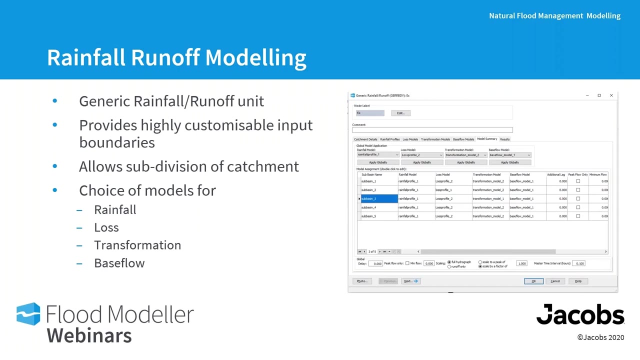 the urbanization, the permeability, or within the individual sub models. you can change things like the initial wetness in the loss model or the timed concentration, the tp in the routine model, to change the behavior of the catchment. worth mentioning is the generic rainfall rough unit. this has been a 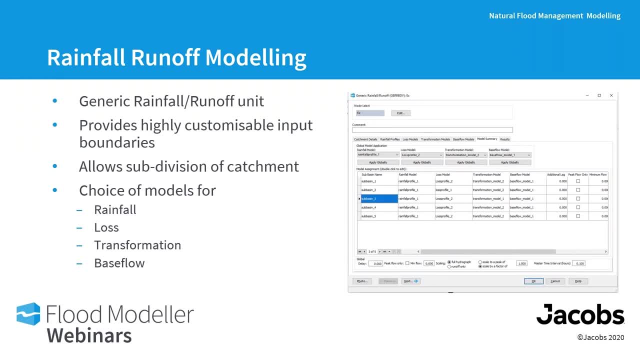 for a long time but has seen some really great enhancements in the last couple of releases. this is a highly customizable rainfall runoff boundary that allows you to change which type of models you use for each component. so your rainfall loss transformation and base flow model. you've got several options. you've got green amp, you've got scs and others. 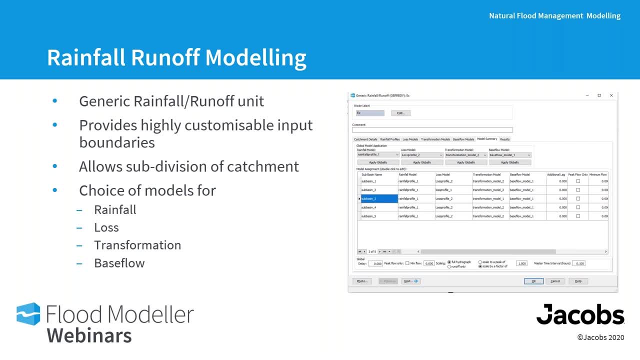 and you can mix and match different components to best represent your catchments. you can also now subdivide your single unit into sub catchments. so an example: on the right hand side i've got five sub catchments and for each one i can specify the rainfall loss, transformation and. 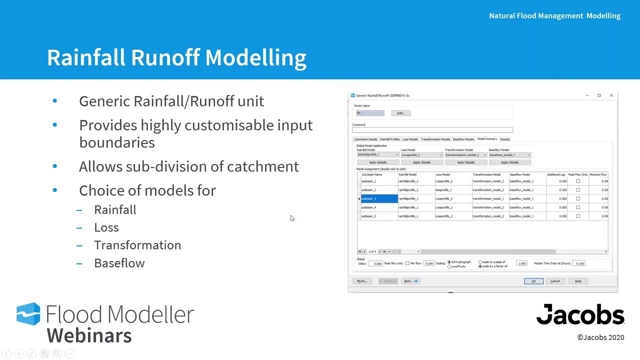 base flow model to represent quite complex large catchments within a single flood modeler unit and then go on to adjust these to represent nfm interventions. if you've not used the generic rainfall runoff unit, i'd suggest you go and have a look at it, because it really is quite powerful. 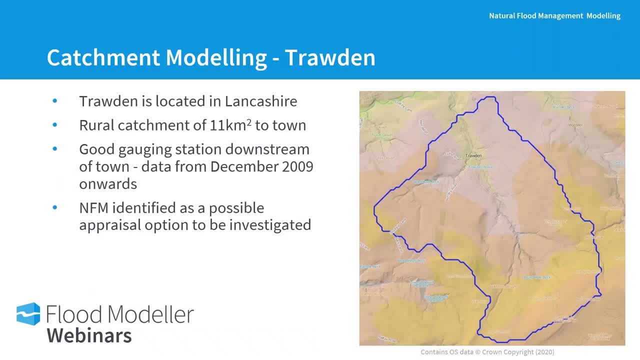 so, moving on from a conceptual approach, looking at more explicit modeling, this is a catchment modeling a place called traudan, where we presented this, uh, this example, a few years ago at a modeling conference. uh, this is where we've used a 2d model to model the entire catchment. 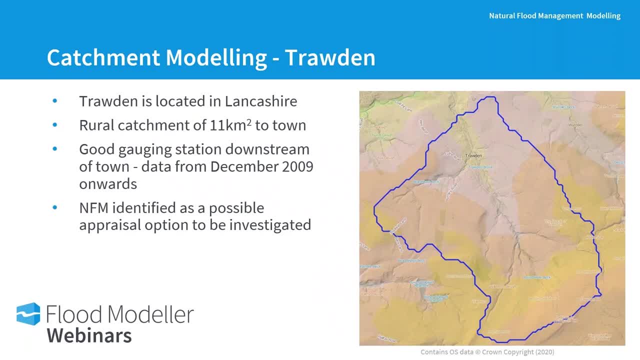 so traudan's up in lancaster in lancashire, up in the uk. it's a rural catchment of actually 11 square kilometers down to the town at the bottom of the catchment and the great thing about this example is there's a gauging station downstream of the. 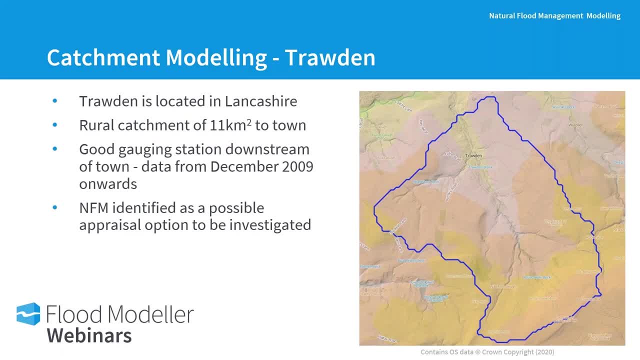 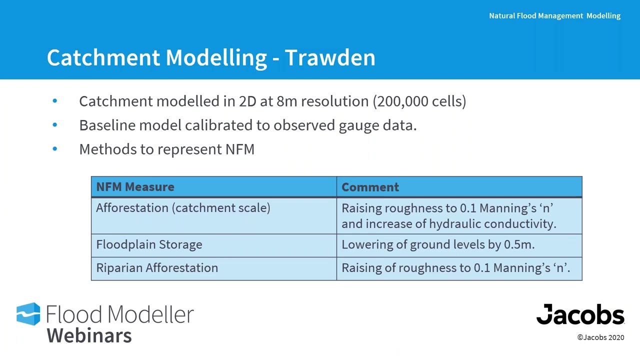 town with a good long record for about 10 years. data to allow us to calibrate the model and nfm needs to be investigated as part of an appraisal of blood risk management options. let's say, a 2d model was built to the whole catchment at an 8 meter resolution. so about? 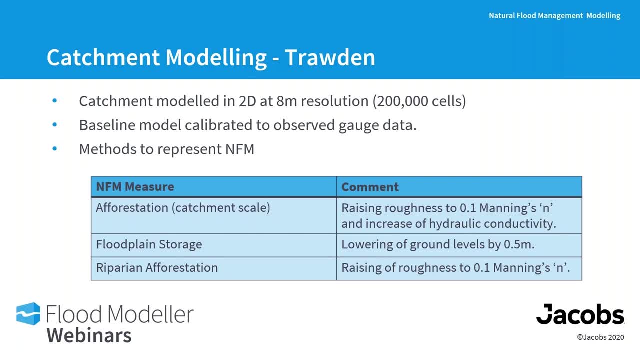 200 000 cells, which is quite a modest size model. now, the important thing here was: the model was built, direct rainfall was applied to the the model and then the various catchment processes were accounted for. within the 2d models we had infiltration, overland flow and such like, and 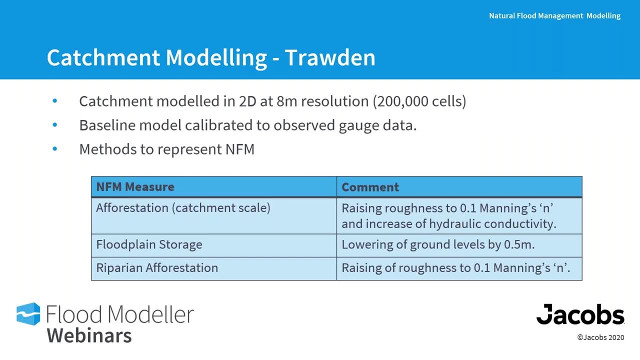 we calibrated the baseline model against that gauge so we had good confidence that the baseline model was responding as the catrin wood and it was a good uh tool to evaluate nfm. once we had that uh calibrated 2d model we could go on to represent different nfm. 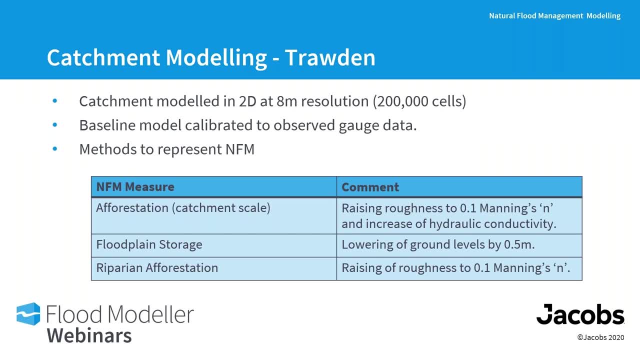 interventions in different ways. um, there's a whole host of these done, but i've picked out a handful. so large scale- a forestation, for example, was modeled through increased roughness, so increasing the surface roughness, the manning's values in the model, as well as increasing infle. trainingereal efficiency prior to protection from aging in the building, which is delicious, manning's values in the model, as well as increasing infiltration range in the building, which is pretty expensive. so anisseil naturalбуldcape with an��릴게요, such as you can see in the page, are 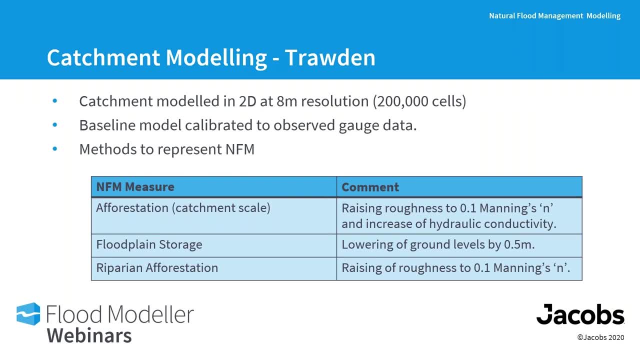 increasing infiltration into the ground. floodplain storage, offline floodplain storage- was modeled by depressing the ground level, so lowering the dtm, in this case by half a meter to represent large areas. offline storage and things such as localized forestation, so localized tree planting, was modeled by increasing the roughness values within the 2d surface. we also consider things such as peatland. 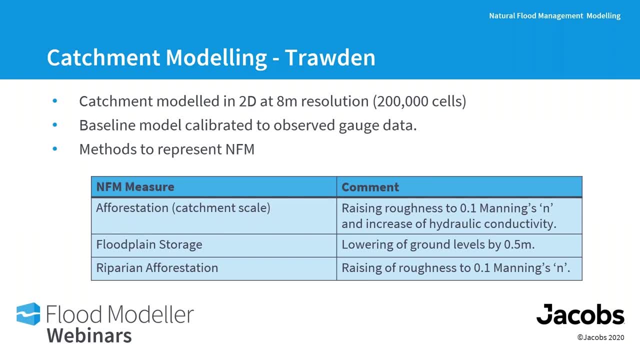 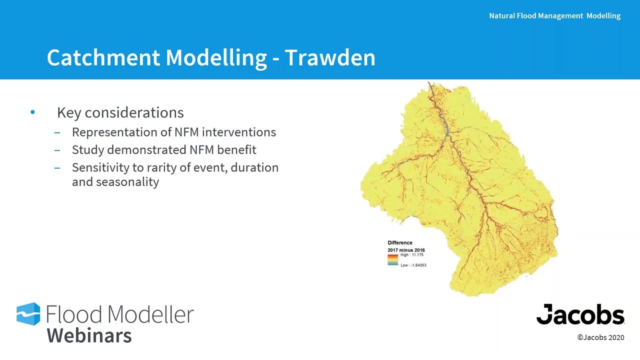 restoration, leaky dams and a whole host of other options all within this one model, and this allowed us to test different interventions and see how beneficial they were downstream. key things that came out from this study were: it was a good study to test different nfm intervention options and how we model those, testing different ways of modeling these things. 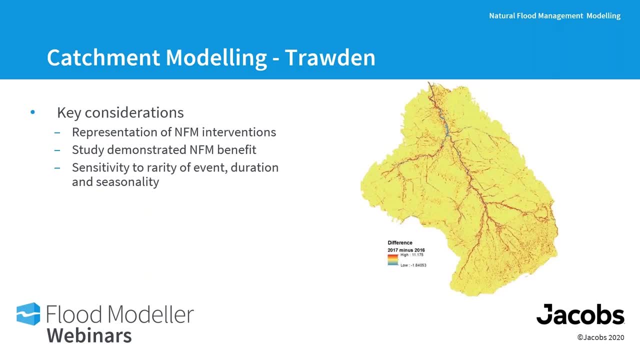 and it clearly demonstrated a benefit to nfm. so we did reduce the flows in the channel but the benefits were very sensitive to the rarity of the event. so with the more extreme events the benefits reduced and also the benefits were very sensitive to the duration and the seasonality of the rainfall events applied. 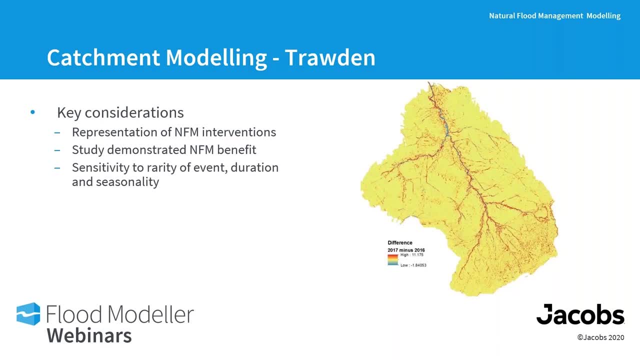 so as we looked for longer wetter winter events, the benefits reduced as the catchment wetted up and the antecedent conditions were such that the nfm interventions had less benefits. so it's important to consider a wide range of different storm events, durations and seasonalities when you do this sort of modeling. 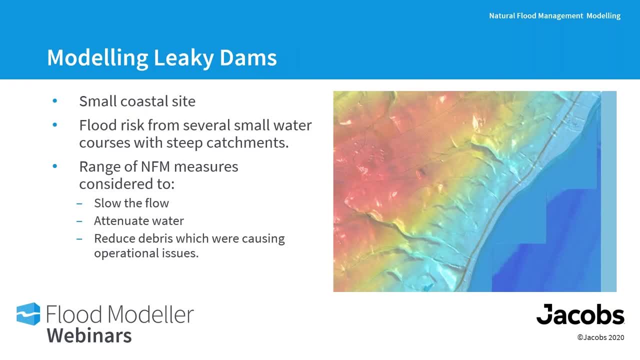 so we've got a lot of different approaches to this model, moving away from catchment based approaches. you can also look explicitly at modeling options. so this is an example where we've got leaky dams being modeled. this is a site where we've got- you can see- the lidar. on the right hand side we've got a very steep hilly area to the west. 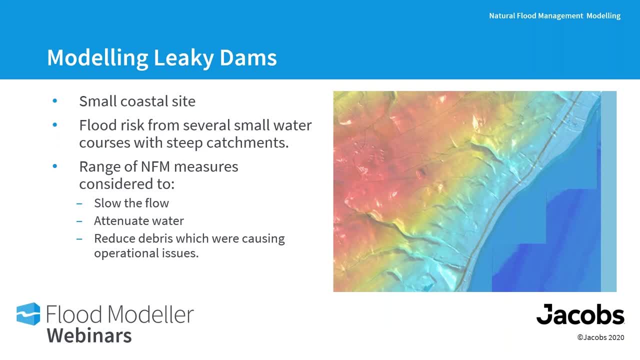 of our site running down into the coast and we're getting high velocity flows coming down a number of channels into our into our area and that was taking high flow but also bringing a lot of debris from the wooded areas upstream. so that was causing flood risk, both from the volume of water coming down the hill but also the debris was getting entangled. 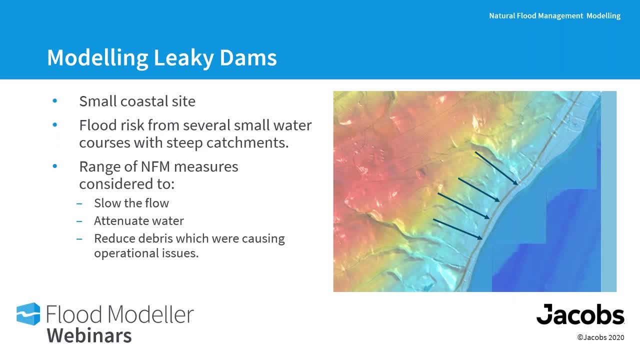 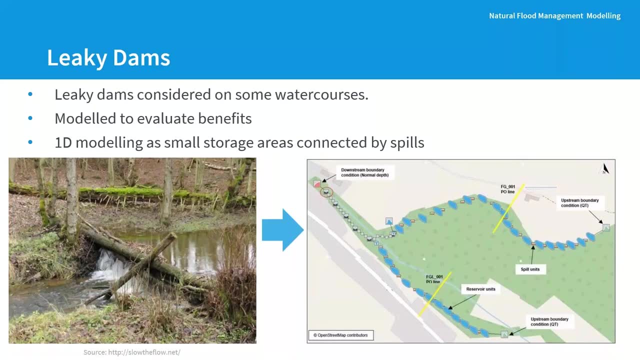 in trash screens causing risk. a number of options were considered to reduce risk and one of those was looking at leaky dams and they were modeled explicitly so leaky down- there's a nice example on the left hand side- is doing a number of things there. it's creating a head loss across it. so getting attenuation upstream with the leaky dam. 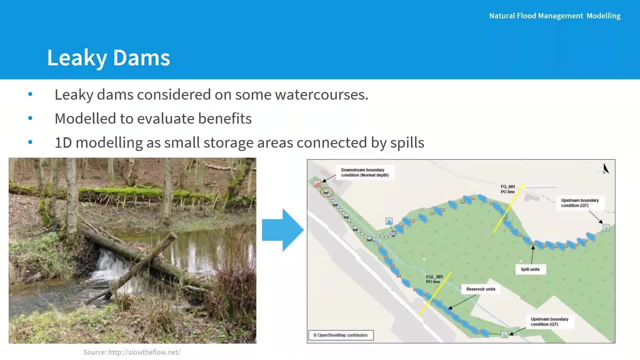 it's also trapping debris, so it's reducing amount of debris being washed downstream and slowing the the rate of flow in the river, and we wanted to model that explicitly in 1d on the right hand side. this is an example of how that could be done. in this case. we had a whole series of these leaky. 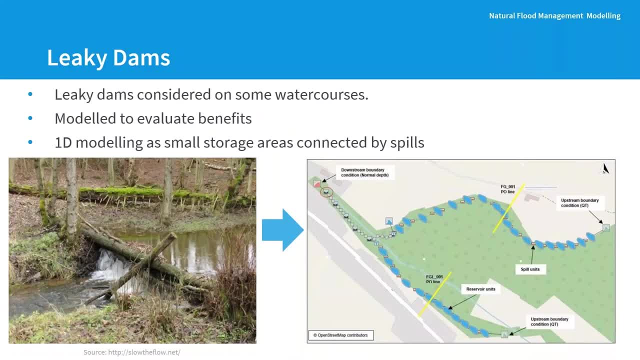 dams being modeled and they were modeled as storage areas, 1d reservoirs in flood modeler and each reservoir was linked up using spill units. so we've got that cascade of leaky dams in our system and this allowed us to evaluate the the benefit of those leaky dams, how much flow they could attenuate. 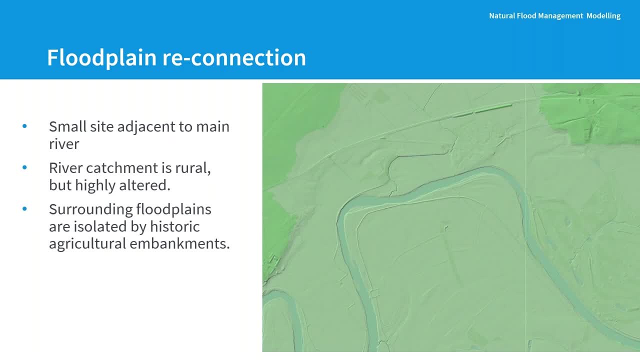 another example is floodplain reconnection, and this is- this is natural flood management, but we've been doing this for a long time as a method for managing flood risk. i've got an example here of a rural catchment where we've got a barrier to flow, so in the center you've got the river. 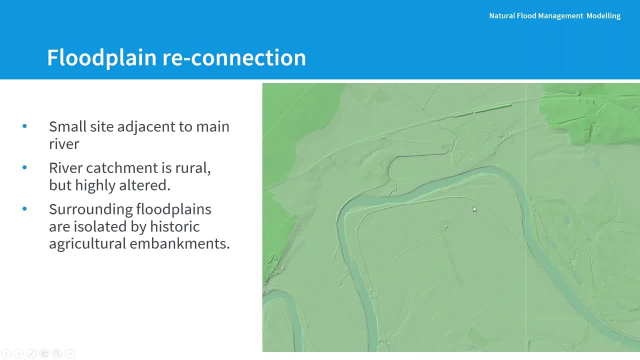 flowing through the area, we've got a large, broad floodplain, and then we've got an agricultural floodplain, and then we've got the river flowing through the area and we've got the river flowing through the area and we've got the river flowing through the area and we've got a large floodplain. 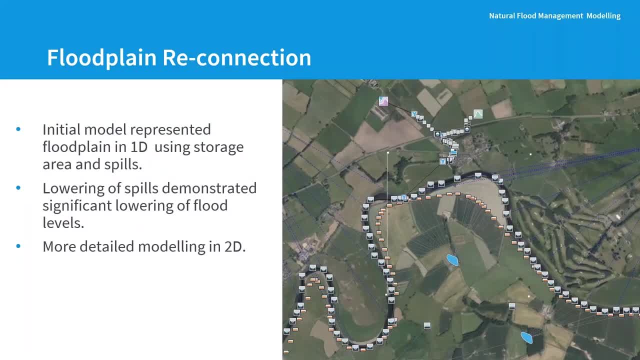 connecting the river, which is disconnecting the floodplain from the river, and so what we want to do is look at the benefits of removing that embankment. this can be modeled in a number of different ways. initially, this was modeled in in purely in 1d, so we're using 1d reservoir units to 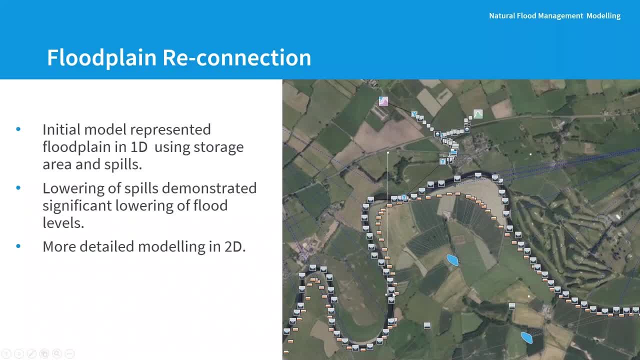 model that floodplain. so you've got your cross sections modeling your channel. you've got a 1d benefits of floodplain reconnection Going a bit further. we could look at that in 2D. So rather than modeling the floodplain in 1D, we could increase the complexity of the 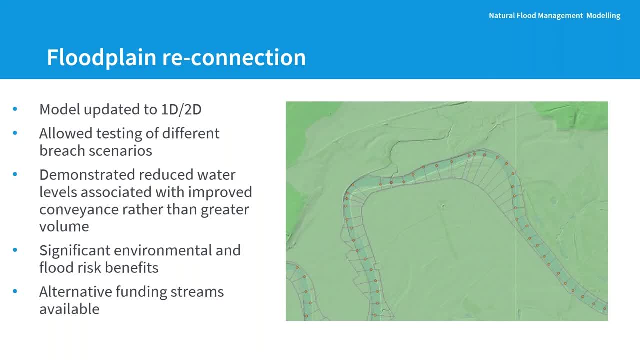 model and model it in 2D instead, So connecting the 1D to the 2D using HX head linking lines, And this gives you a lot more information about how that floodplain responds and also demonstrated that there were significant benefits associated with reconnection to the floodplain. 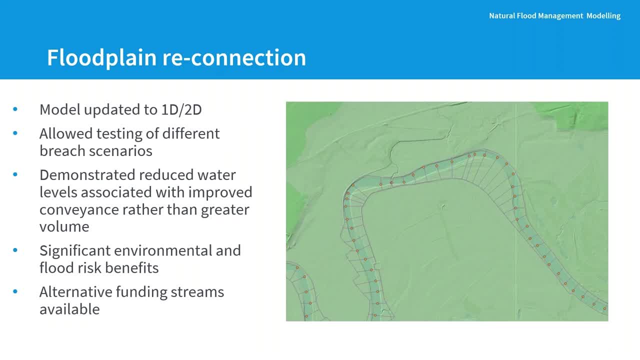 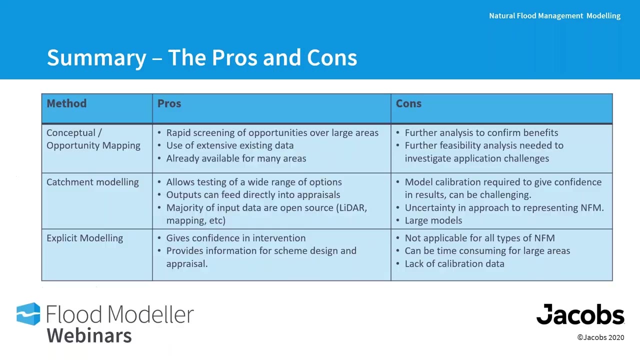 both environmental and flood risk, And by identifying and giving information such as extents and depths of water, we could look at alternative funding streams to fund those options. So by creating new habitat, you can access additional funding streams for your schemes. I've talked about a number of methods there and I just want to touch on the benefits. 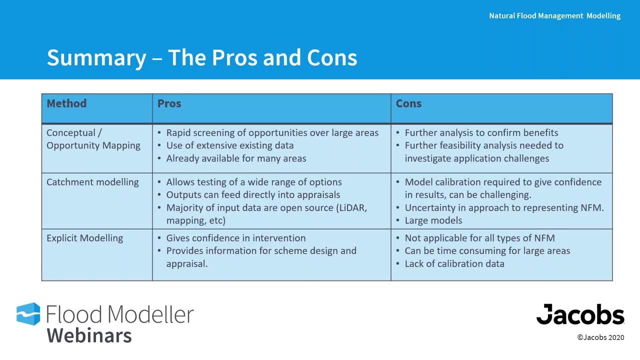 and challenges associated with each one. So the high level opportunity mapping type approach is great. You know you can screen large areas, large catchments very quickly using existing data. But if it's just looking at the existing GIS data, that doesn't tend to tell you much about the benefits of NFM. 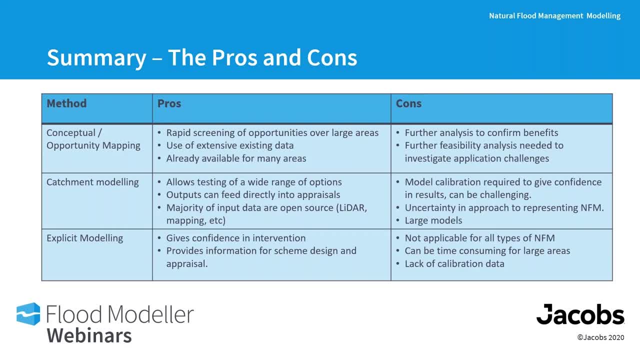 So once you identify the options, you then need to go on and model them in some way to evaluate their benefits. Catchment modeling using conceptual models or 2D models allows you to test a wide number of options in your catchment very quickly and you can take the 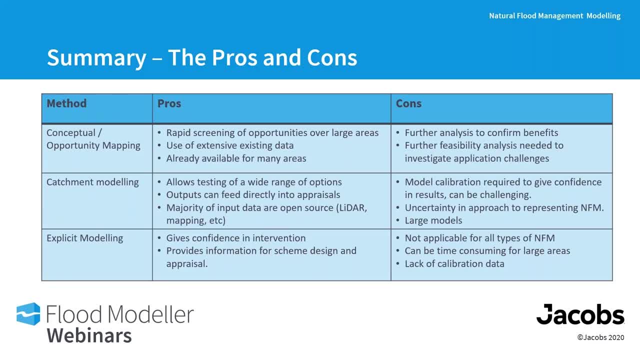 outputs from those models directly into appraisals, And lots of the data is open source so that you can build these things quite quickly using open source LIDAR and mapping data. The key challenge with these are calibration, So you need calibration in the model to give. 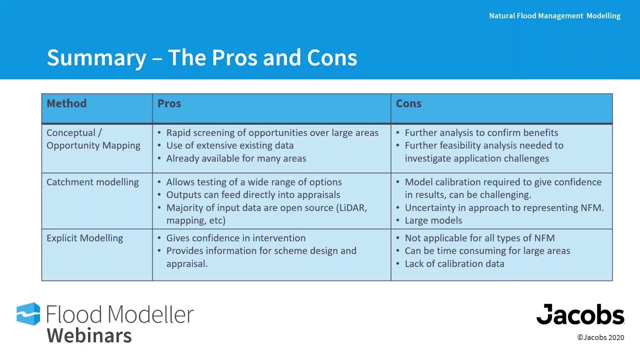 you confidence that they're behaving properly, And there's still a large degree of uncertainty associated with how you represent your NFM interventions. Finally, your explicit models give you good confidence in how your intervention works and provide scheme design information, but they can't be used for all intervention types. 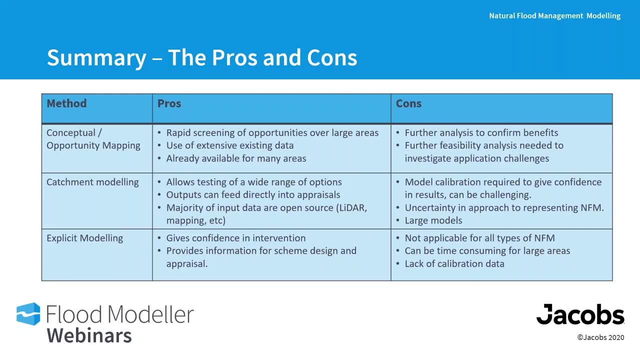 And it can be quite time consuming to set up some of these models. So if you've got hundreds of leaky dams to add, that could take quite a bit of time, And as will the others. calibration information is key. Just to summarize some of the challenges and 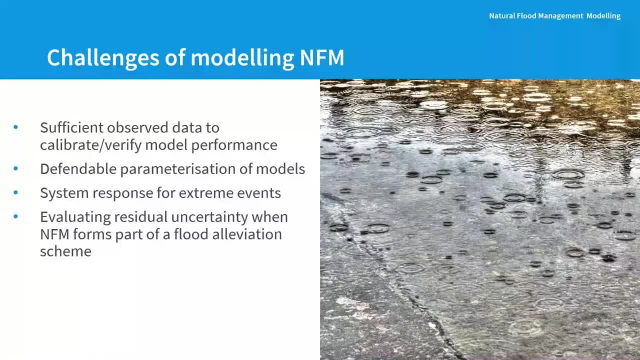 things you should be aware of when you're doing this sort of modeling. sufficient observed data to calibrate and verify your models is essential, as well as defendable parameterization of your models. So if you're making a change to represent NFM, is that defendable? I've 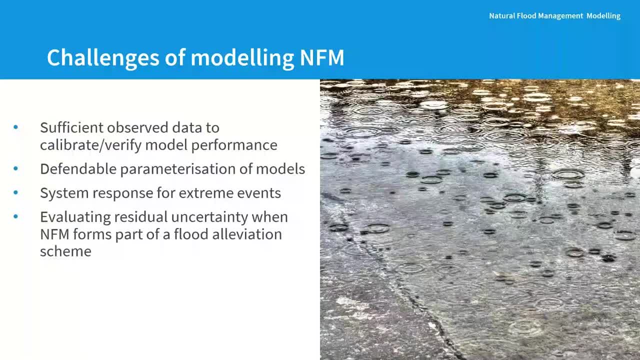 put a load of links at the end of this presentation to sources of information and where you can get information to support your decisions. You need to consider your system response to extreme events. So NFM may work really well for low order events, but do they work so well for long, wet winter events as well? 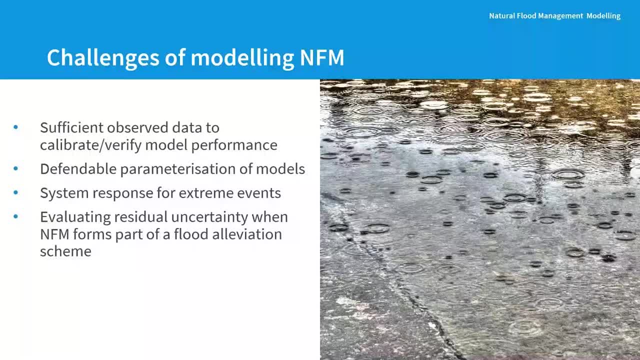 You need to consider the whole number And there's an issue around residual uncertainty. So if you're implementing NFM to provide a standard protection, how much confidence do you have that NFM option is going to work? There's undoubtedly a lot of uncertainty around that. So if you're implementing NFM to provide 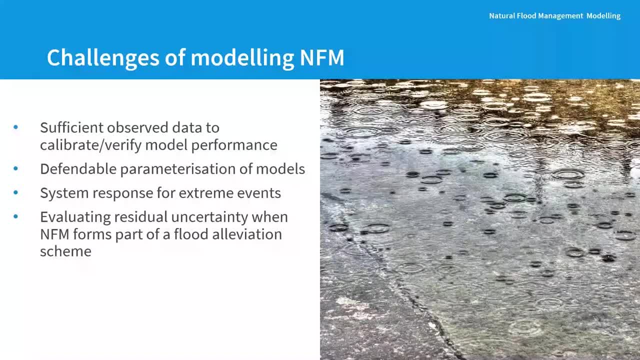 a base reaction: bitter data or photographs which is not interesting or very more involved in projects. that's why we recommend NFM. In addition, our research in the telco and in cloud. 我们希望是融合速度. 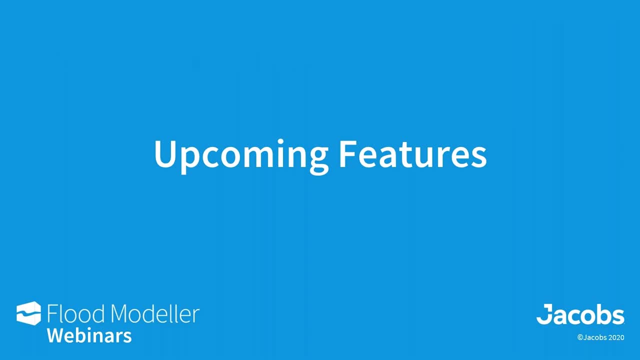 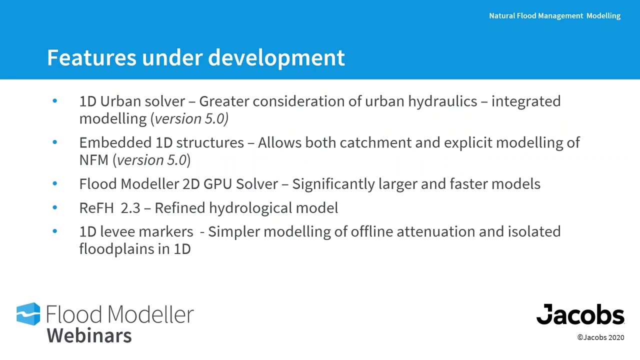 but in the future it's likely to be used to estimate load gap or Issue a greater residual uncertainty associated with it, In addition to the features and the functionality I've talked about of the last 20 minutes. So there's a number of features coming to flood model which should give you greater 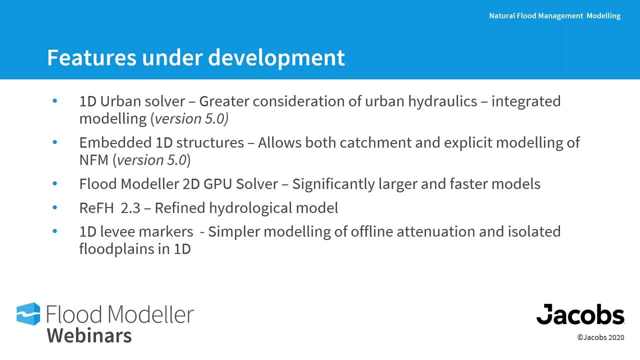 flexibility and how you consider NFM. So the next release has got the one the urban solver. I spoke about urban pipe networks. Also, we'll be having embedded 1D structures, allowing us to put 1D structures directly into a 2D model in a far more simplistic manner. 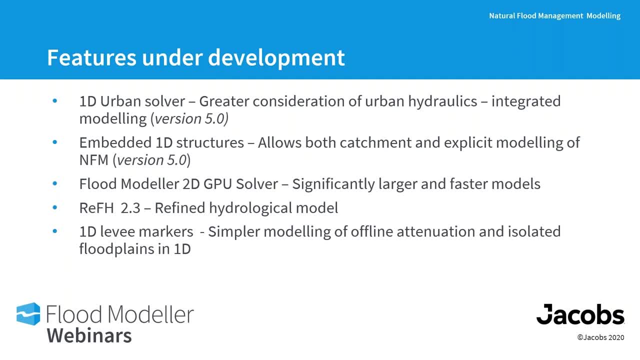 So that opens up options for doing things like leaky dams directly within a 2D catchment model, for instance. Not in the next release, but on the development pipeline. we've got things such as Flood Modeler, 2D GPU solver. 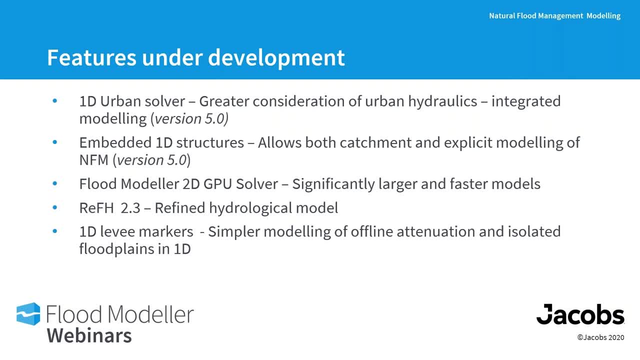 So running our 2D models a lot faster using GPU cards or allowing us to model far larger areas. We've also got the new release of RFH 2.3 and the linking with Flood Modeler, as well as things such as 1D levy markers. 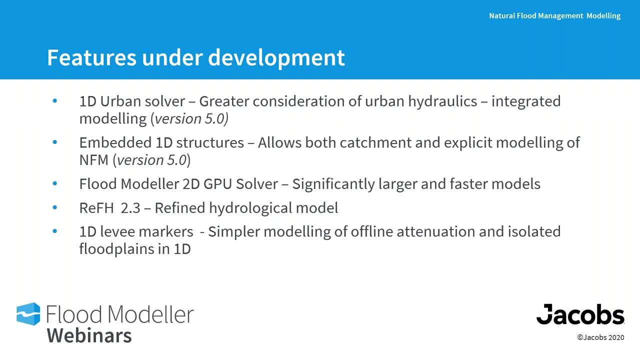 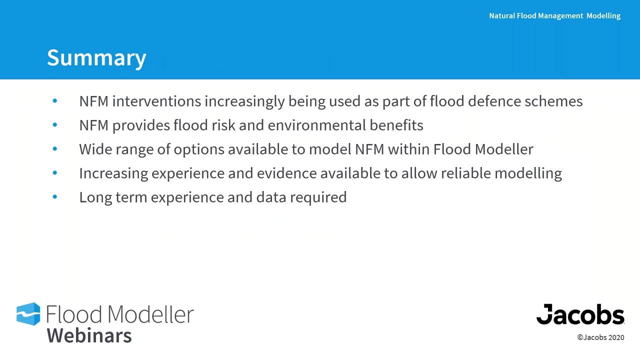 So allowing us to model offline storage, attenuation or isolated floodplains a lot more simply than you currently can. So there's some exciting things coming in Flood Modeler. So just to quickly summarize, NFM interventions are increasingly being used as part of flood defense schemes because they bring both flood risk and environmental risk. 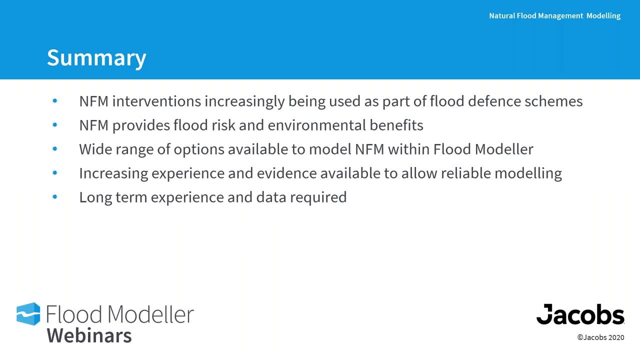 There's a huge number of ways of modeling these within Flood Modeler so you can evaluate the benefits of these NFM options And we've got increasing experience and evidence to allow us to justify and give us confidence in our modeling options. And I say there's some links to that evidence at the back of this presentation when it's published. 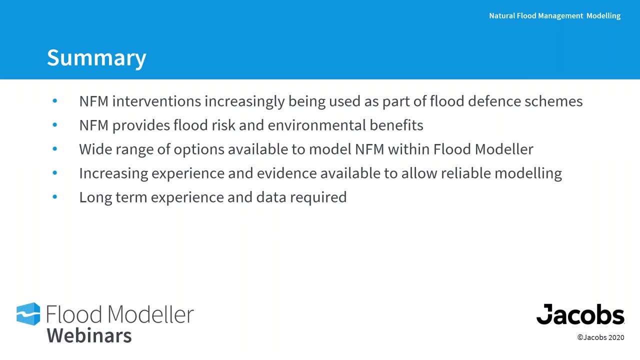 Undoubtedly we need longer term data and experience, so we need to carry on modeling and monitoring these interventions to give us that evidence base to justify our work And to further justify future NFM interventions.